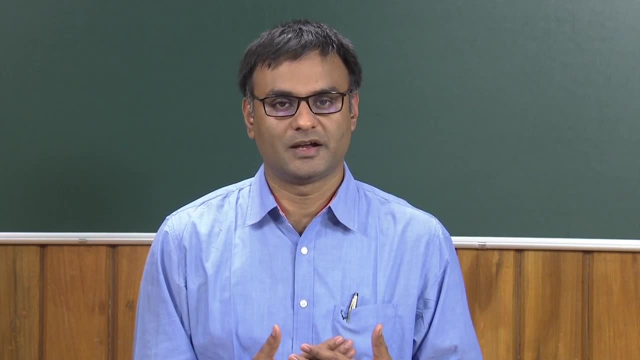 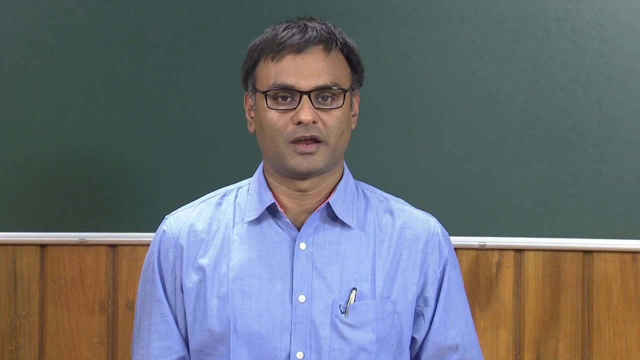 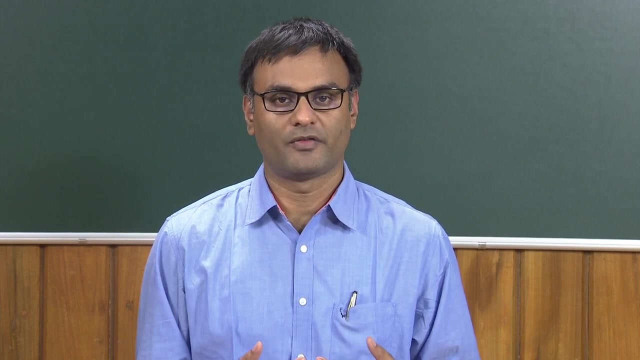 then of course you need to have a good understanding of the cardiovascular fluid mechanisms. So for a biomedical engineer or for a biosciences and bioengineering student, It is important to have an understanding of the flow in cardiovascular system. This course is for about 10 hours and it will be useful for the 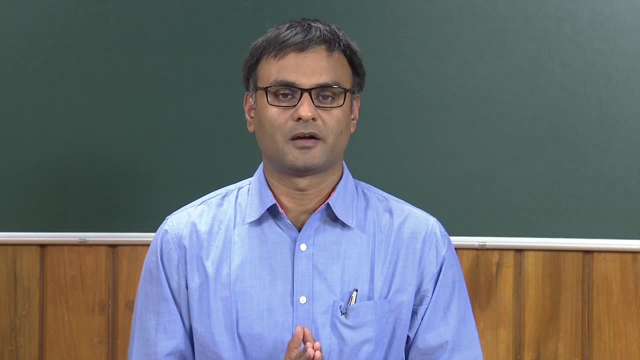 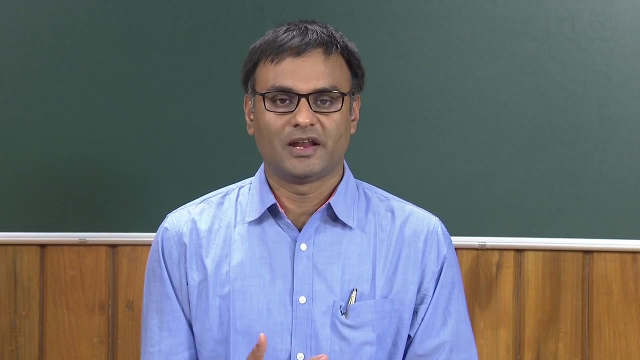 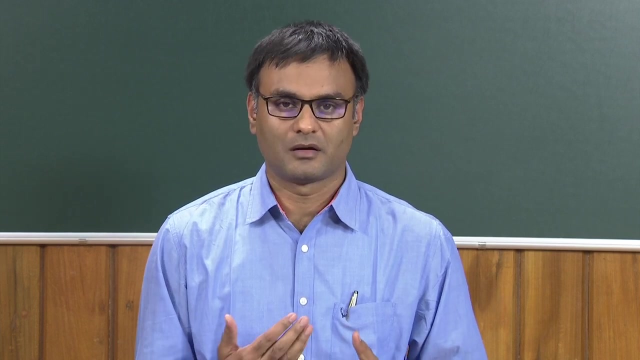 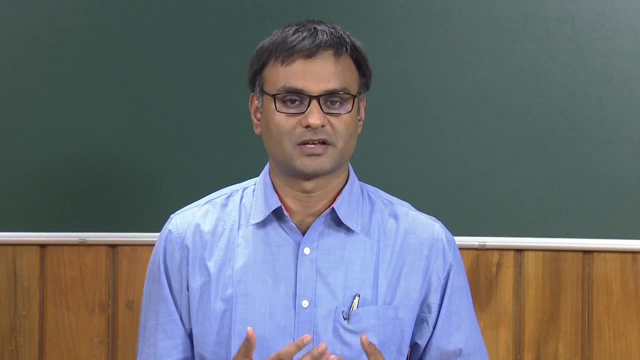 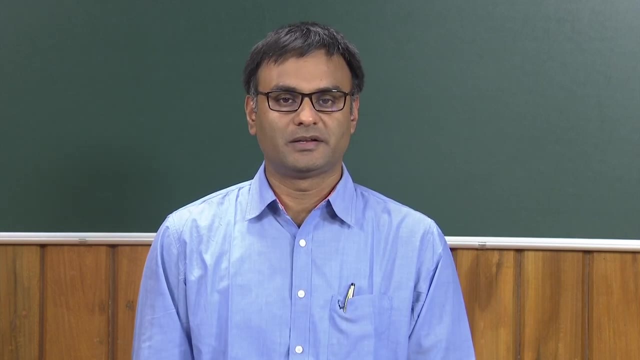 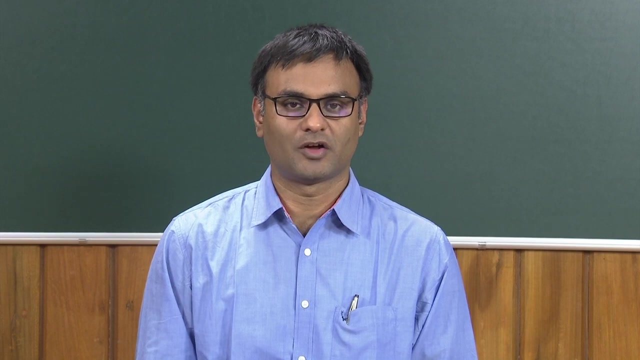 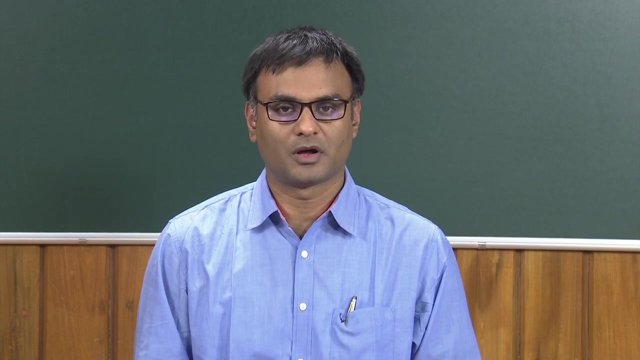 biosciences and bioengineering, so, for example, the students from chemical and mechanical engineering in this course. we expect that the student would have done basic course on fluid mechanics at the undergraduate level of engineering, so he would be familiar with what continuum equations are, for example, what is mass? 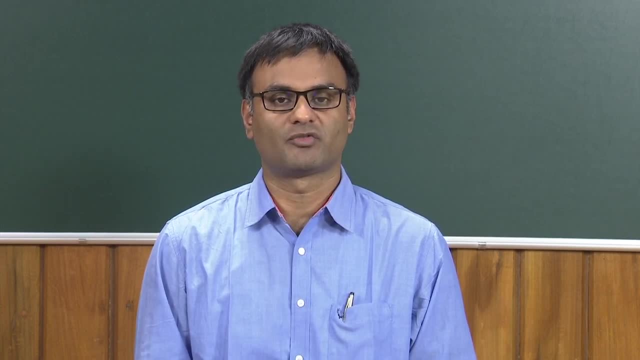 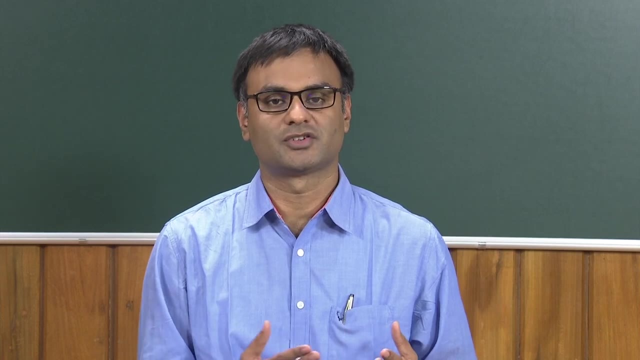 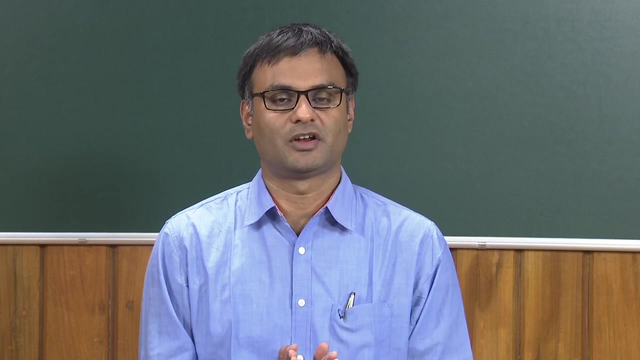 conservation and momentum conservation equations. what is a Navier-Stokes equation? what is flow? a fully developed flow in a pipe? of course, he will also have knowledge of inviscid flow, where, for example, the Bernoulli's equation, where he can obtain a relationship between pressure and velocity, neglecting the 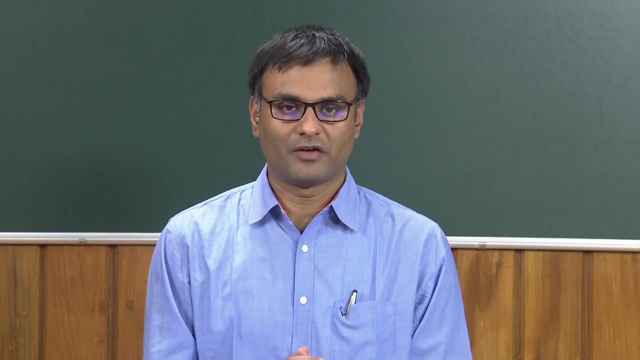 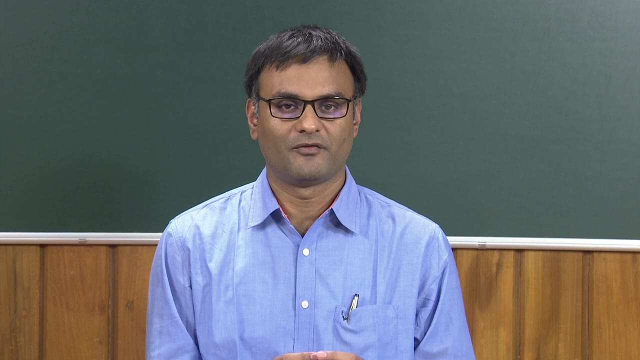 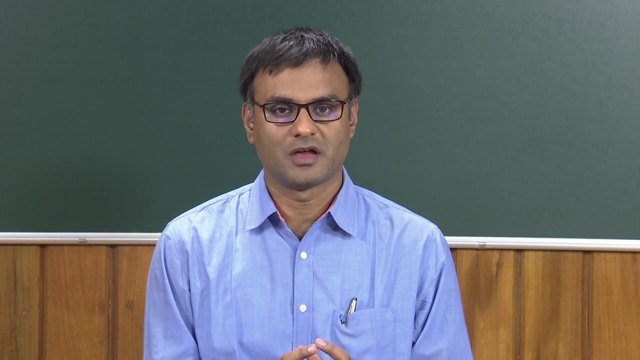 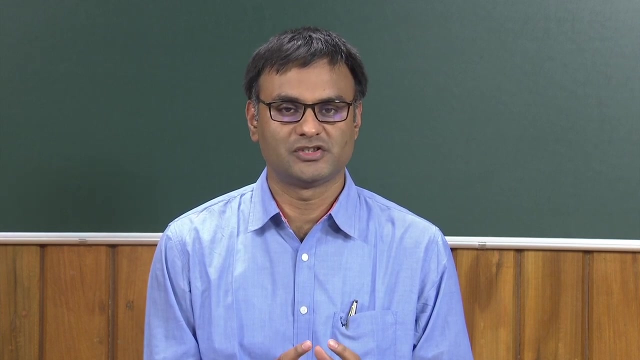 viscous losses. so what this will course cover. the course will quickly talk about the physiological system of cardiovascular system, because that is what we are going to study. so first we need to understand the cardiovascular system, the physiology of the cardiovascular system, briefly. so we need to understand first the property of the fluid that is being 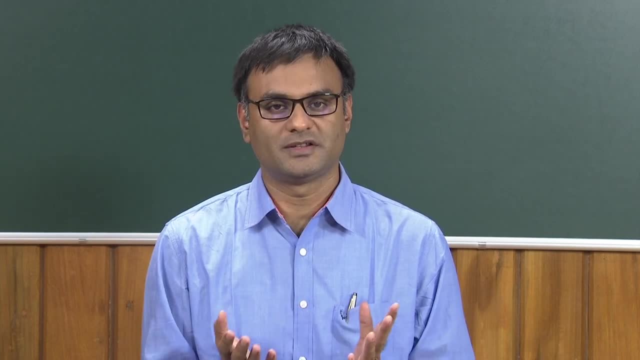 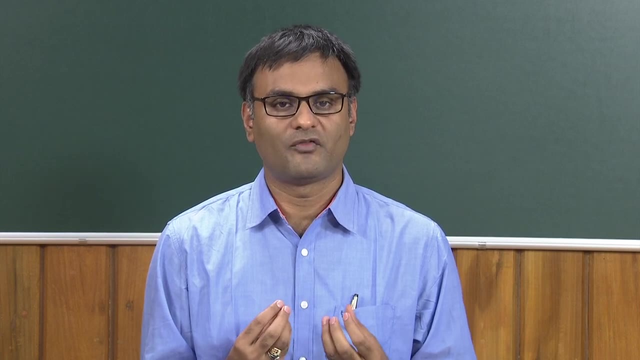 はい. pump and blood is a complex fluid. it has number of flexible particles suspended in ly. so we need to understand first the property of the fluid that is being. pump and blood is a complex fluid. it has number of flexible particles suspended in it- white blood cells, red blood cells and platelets- and their volume fraction is 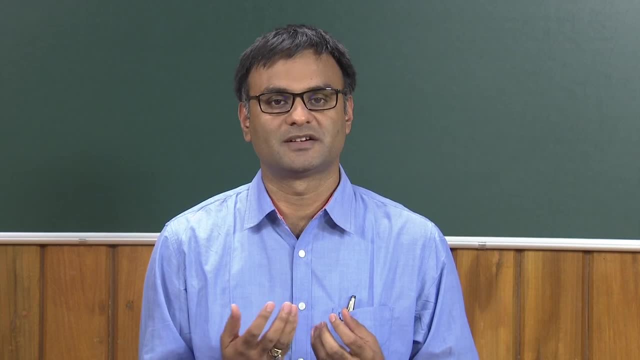 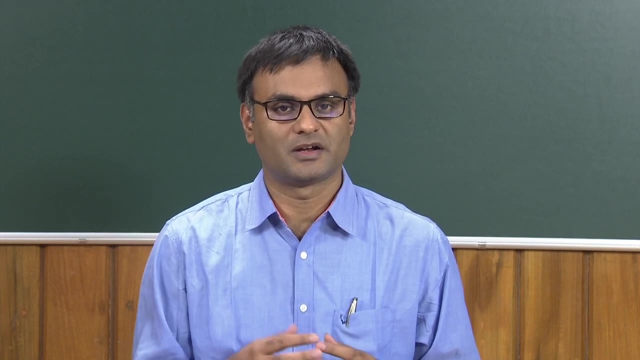 moved and is about fifty percent in, and they are suspended implant one. so we need blood cells and platelets and their volume fraction is about fifty percent in. understand the particular biology of blood. biology falls under the zelf non- dips. we also understand transverse general스�, injuries, blood doctors and researchers. 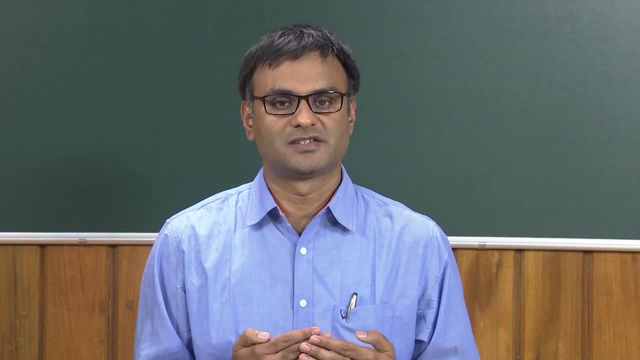 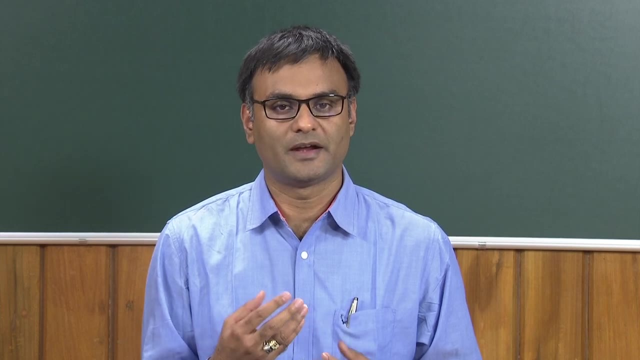 as well as hyperl파 Broadway campus ici, and it is partly because even I said that lia john's problems for cardiovascular system, so there are some problems. this is not a considerable need to understand. so for those people who have experienced the is basically the relationship between stress and strain rate. that is, when a force is applied. 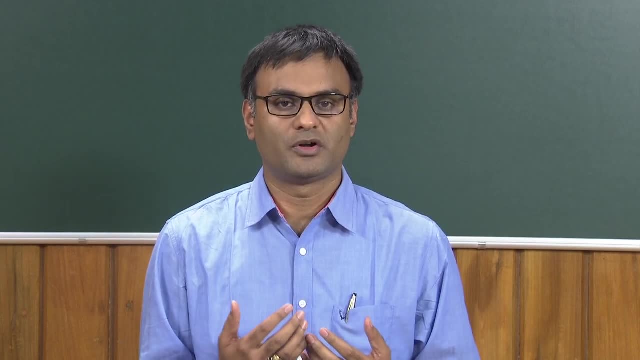 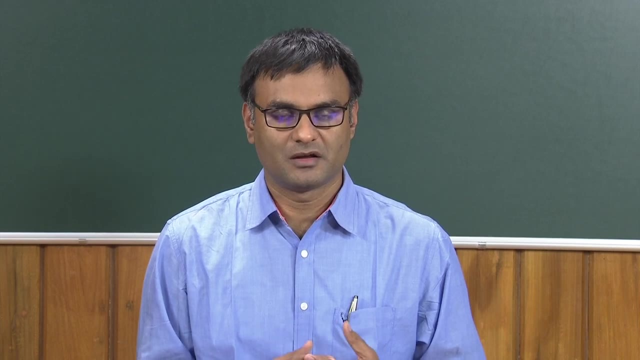 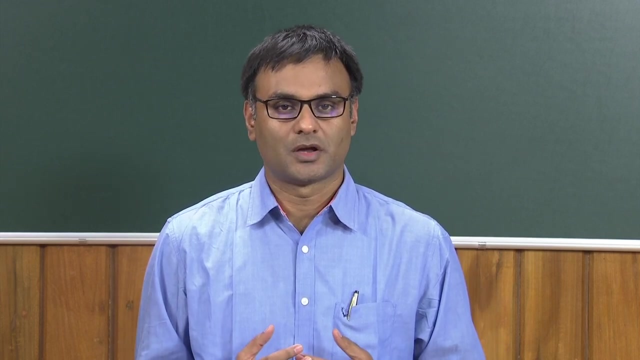 on a fluid, how does it respond to it? what is its rheological or flow behavior? So that is the first thing that we will study: rheological behavior of blood. Then we need to understand the pipes, or the piping network, which is arteries and veins in this case. 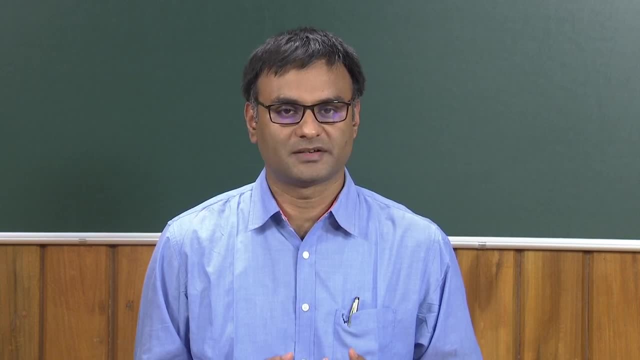 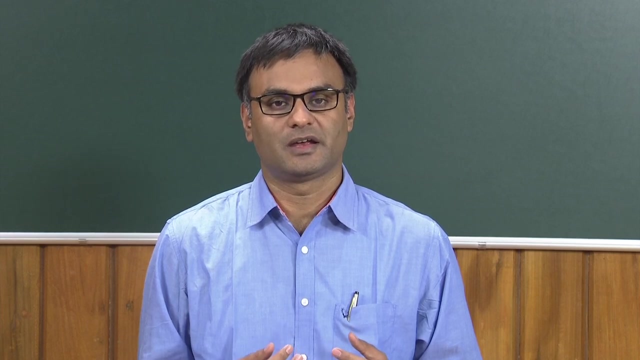 what is the properties and characteristics of those? So, as you can guess that the arteries and pipes, or arteries and veins in which the flow happens, they are not the rigid tubes As we generally consider in a conventional fluid mechanics course. so one need to take. 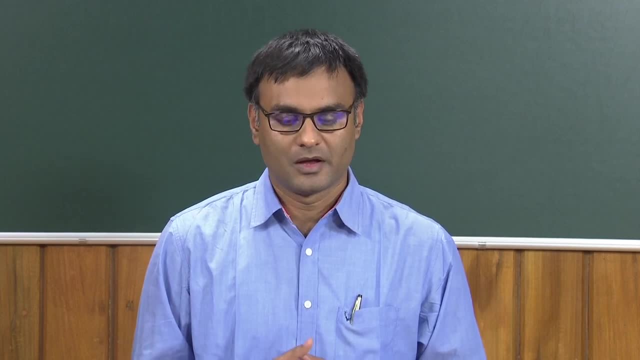 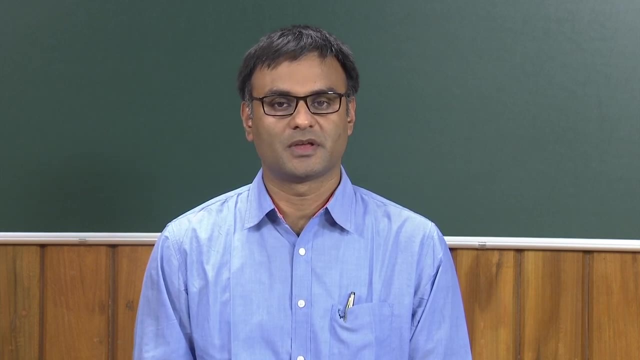 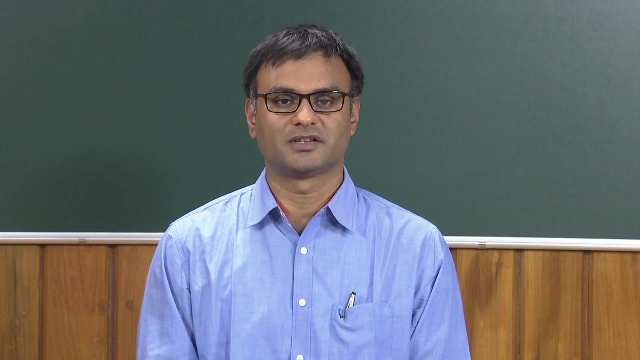 into account the flexion Flexibility of pipe, plus the another complexity, or another point that is different in the cardiovascular system is that the flow is not steady With. this is not the case in a cardiovascular system, because the flow is pulsatile and we need to understand the pulsatility. 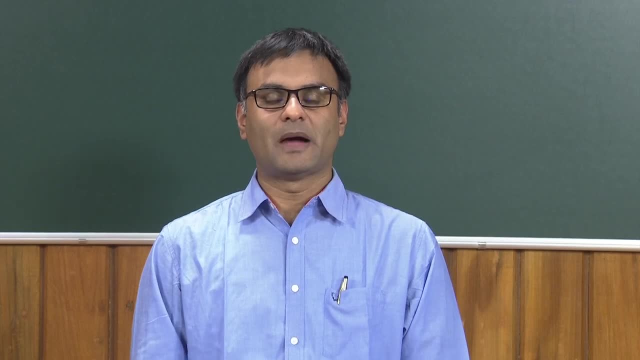 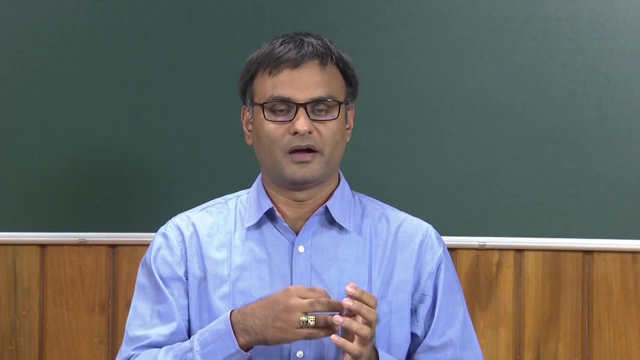 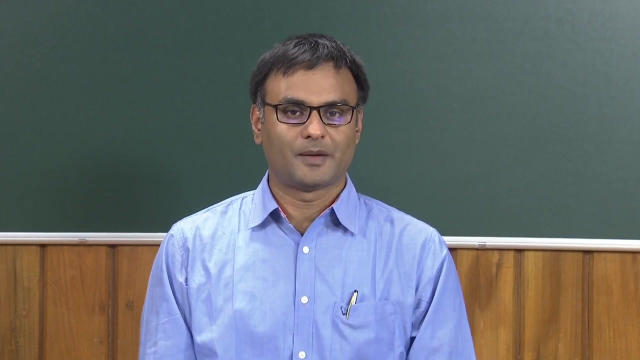 of the system, Then the flow bifurcates several times. the flow comes out of heart and from there it comes to a aorta or a bigger artery and from there it bifurcates into different parts of the body. So we need to understand the bifurcating flow and the effect of curvature. 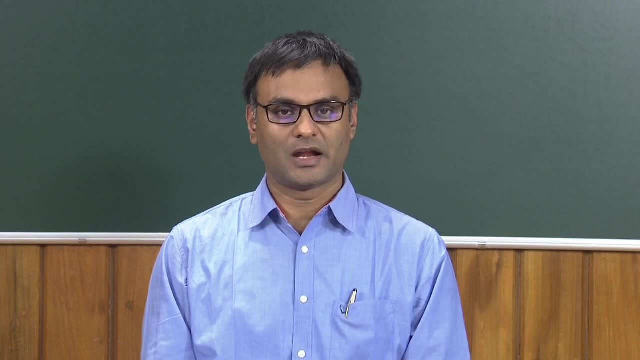 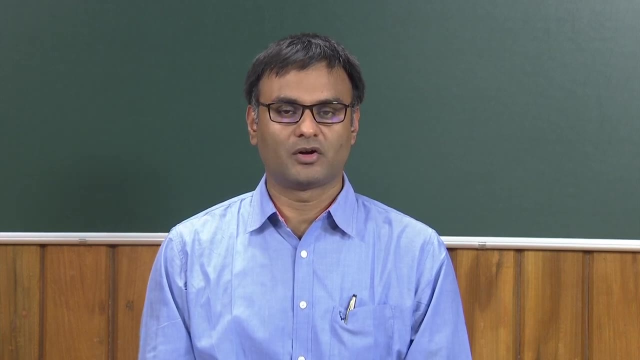 So these are some of the topics that we will cover in this 10 hours lecture. Hope you would be able to learn and try to understand or try to apply by the end of this course. try to apply the fluid mechanics concept To understand the biological system. Thank you.